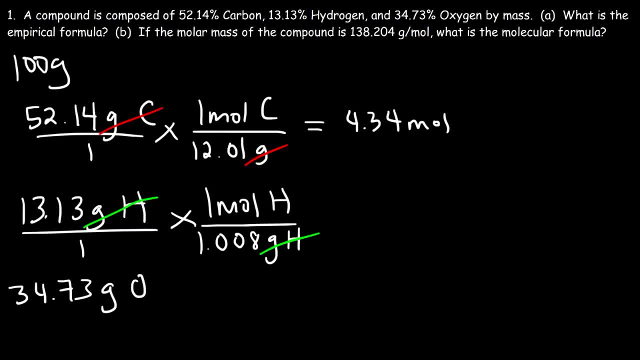 So let's take 13.13 and divide it by 1.008.. So this will give us 13.026 moles of hydrogen. Lastly, we have oxygen, The molar mass of which is 16 grams per one mole, So 34.73. 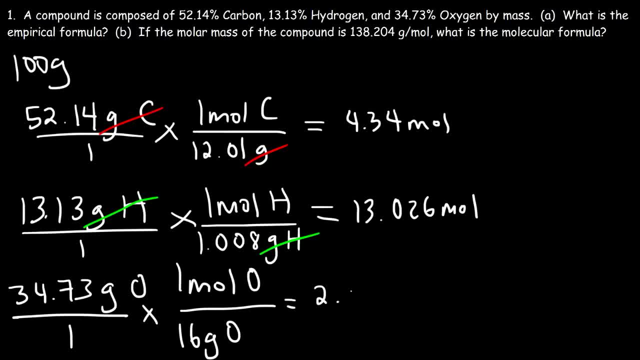 divided by 16. That's 2.171 moles. Now what you need to do next is identify which number is the smallest. Clearly, it's the moles of oxygen, So what you need to do is divide every quantity that you have, So, in this case, En MINT. 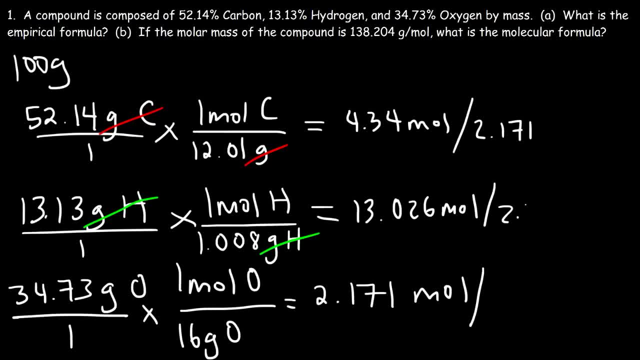 by the smallest of the 3 values, In this case the moles of oxygen. Ideally you want to get a whole number, 4.34 divided by 2.171.. That is aboutIt's 1.999mol, if possible. 13.026 divided by 1.65ب, It is 1.'899.. 141.하다, That's 1.9999.. 13.026 ÷ 2.171.. ambitions 159.. llegao para Ε 14.904 di wawakita, ее 14. 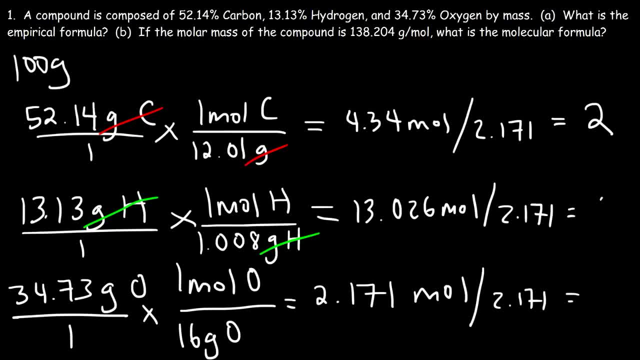 two point one, seven. one is six and this is clearly one. so now we have the subscript for carbon, the subscript for hydrogen and the subscript for oxygen. so the empirical formula, that is the formula with the lowest ratios. it's C, 2, H, 6, 0, 1. so that's the empirical formula. that's how you could find it, if you're. 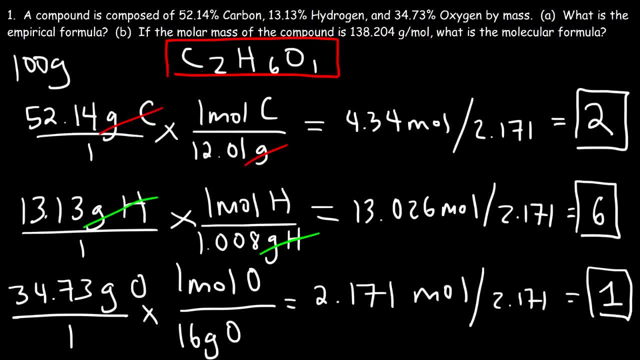 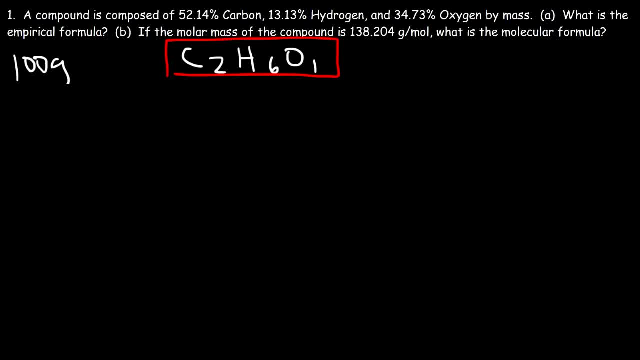 given the percent composition of an element. so that's the answer for part a. now let's move on to part B. if the molar mass of the compound is 138 point two zero four grams per mole, what is the molecular formula? so we have the empirical formula. now we need to find the molecular formula, the first thing we 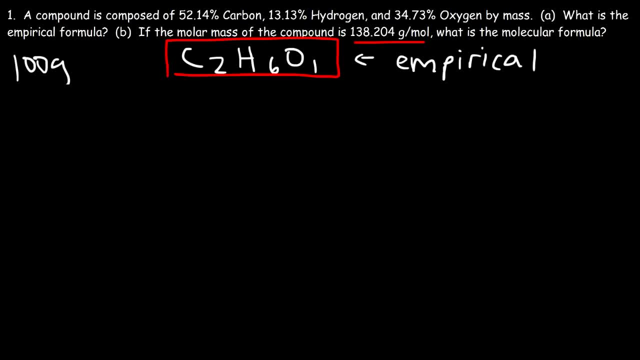 need to do is find the molar mass of the empirical formula. so there are two carbons, six hydrogens and one oxygen. so it's two times 12.01 plus 6 times 1.00, 8 plus 16, so the molar mass. 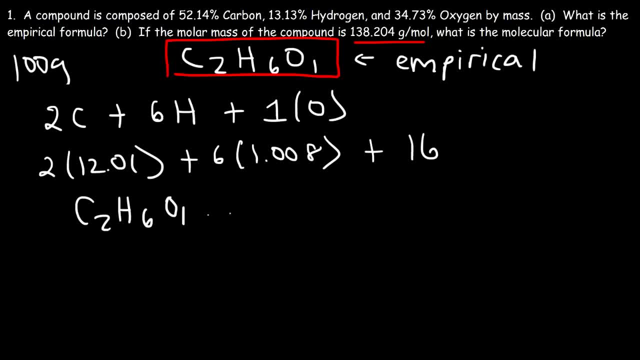 of C2H6O1 is 46.068.. So now we need to know what empirical formula, or rather what molecular formula, corresponds to a molar mass of 138.204.. So what you need to do is take the larger number. 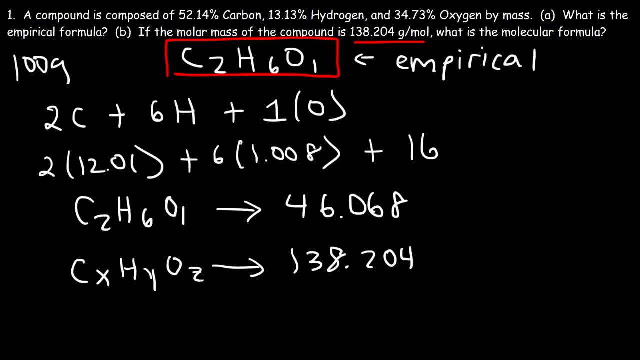 and divide it by the smaller number. So if we divide 138.204 by 46.068, we are going to get 3.. So if you multiply 46 by 3, you get 138.. So therefore, to get the molecular formula. 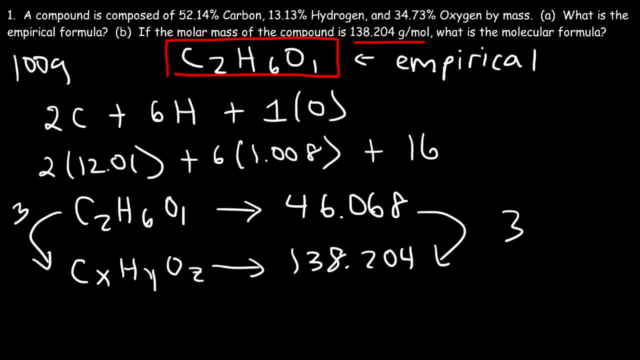 we need to multiply the subscripts of the empirical formula by 3.. So this is going to give us C6H18- O3.. And that's how you find the molecular formula from the empirical formula. Basically, you got to divide the molar mass of the molecular formula by the molar mass of the. 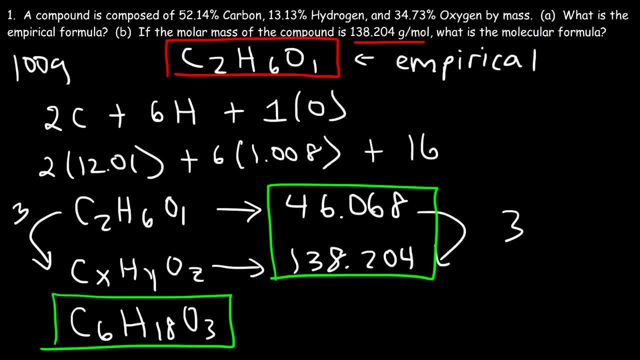 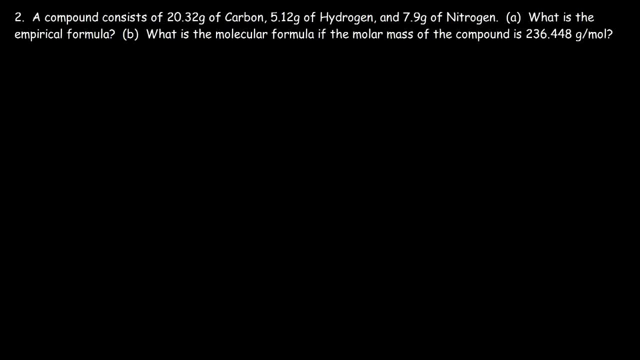 empirical formula. Whatever number you get, multiply the subscripts of the empirical formula by that number and that's going to give you the molecular formula Number two. a compound consists of 20.32 grams of carbon, 5.3 grams of carbon. 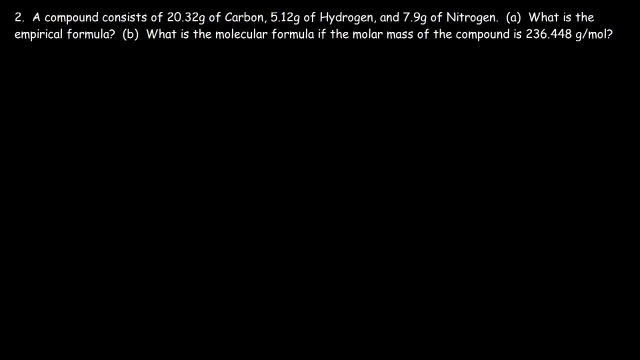 5.3 grams of carbon, 5.12 grams of hydrogen and 7.9 grams of nitrogen. What is the empirical formula? So in the last example we were given a percent composition, which we converted to grams anyway. 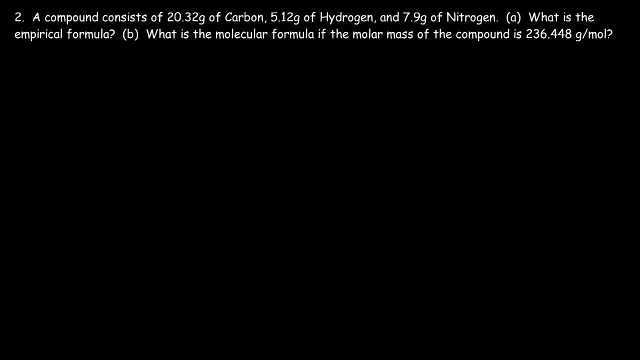 Here we're given the grams of all the elements in this compound, So we're going to follow the same steps of converting each into moles. The molar mass of carbon is 12.01 grams for every one mole of carbon. 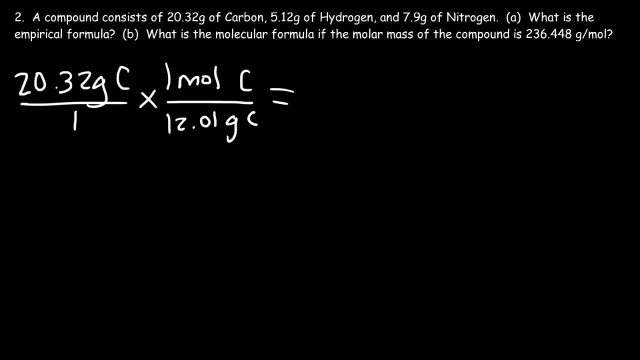 So 20.32 divided by 12.01, that's 1.692 moles of carbon. So now let's turn our attention to hydrogen. The molar mass is 1.008 grams of hydrogen per one mole. The molar mass is 1.008 grams of hydrogen per one mole. 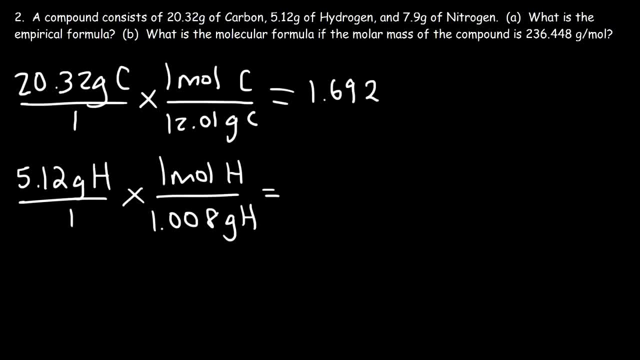 and so this is going to be 5.079. and finally, let's move on to nitrogen. we have 7.9 grams of nitrogen, and the molar mass is 14.01, so this will give us 0.5639 moles of nitrogen. so now let's divide each number. 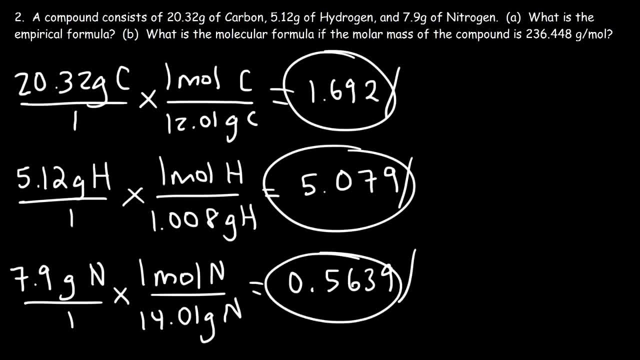 by the smallest of these three values. so the smallest is 0.5639. so 1.692 divided by 0.5639, that's about three. 5.079 divided by 0.5639, that's nine, and this is going to be one. so in the empirical formula there, 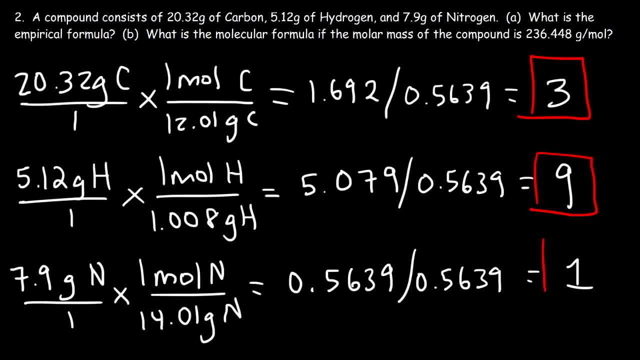 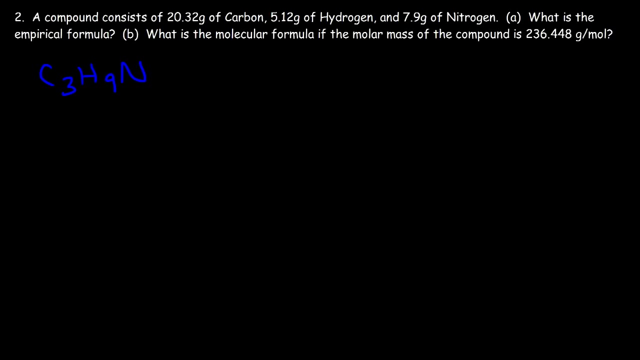 should be three carbon atoms, nine hydrogen atoms, one nitrogen atom. so the formula is going to be C 3, 3H9N1, or simply just N. So that's the empirical formula. Now let's find the molecular formula. To do that, we gotta find the molar mass of the empirical formula first. So we have three.